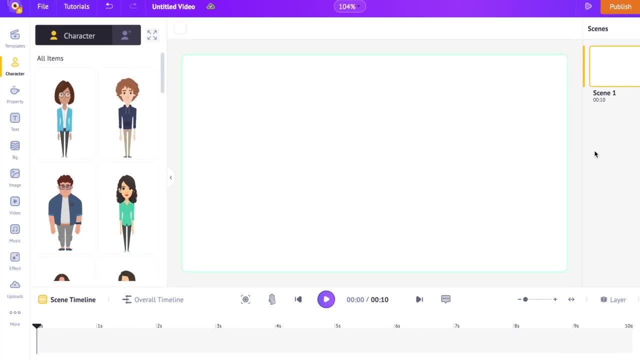 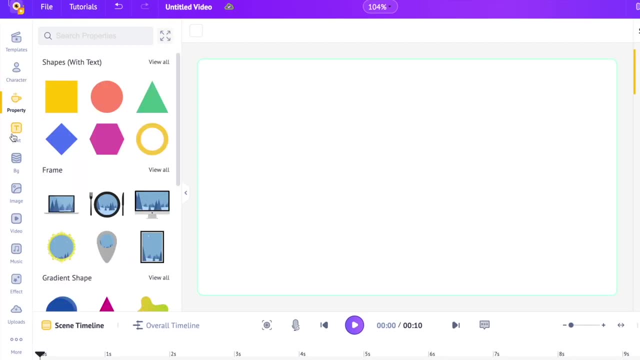 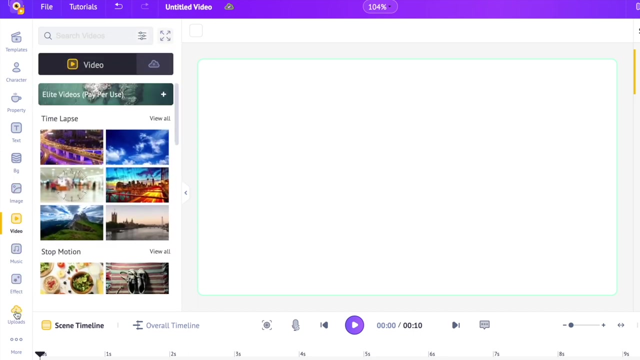 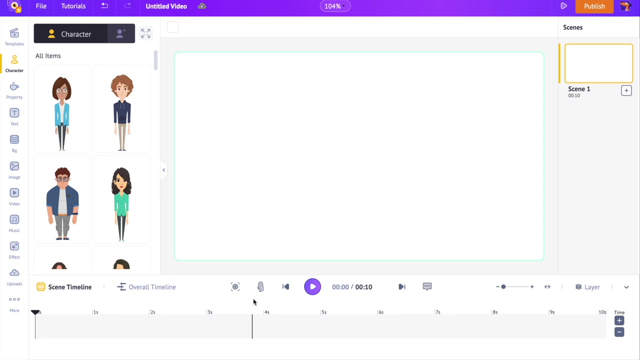 scenes together form a video. On the left hand side is the library. Here is where you can find elements like animated characters, illustrations, backgrounds, images, videos, music tracks that will be needed to create a video. The bottom is the timeline. Here's where we'll be editing and customizing the elements that will 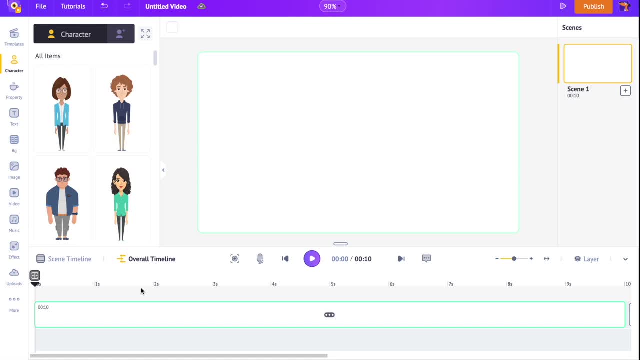 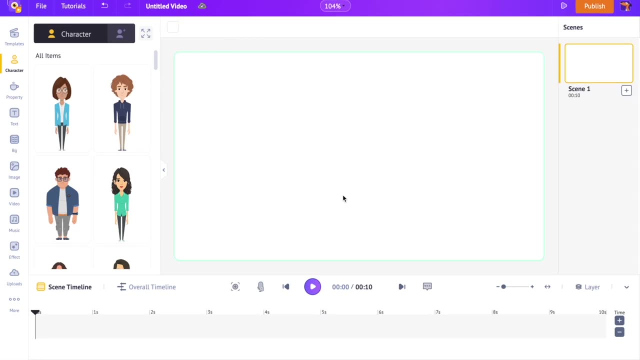 appear on the video. It is further divided into scene timeline and overall timeline. Let's start with adding the character to the scene. We have two options in selecting a character. Either we can select a character from the library of Animaker or we can create a character from scratch. If we look at the library, it has a variety of 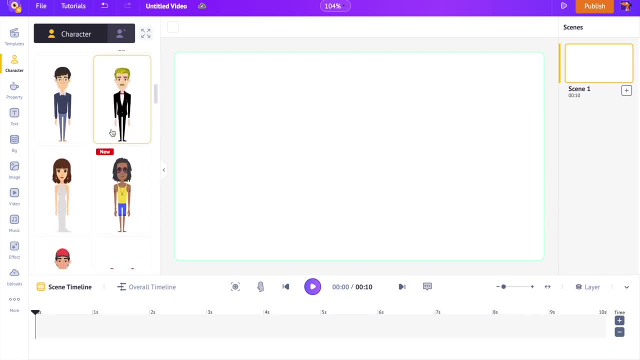 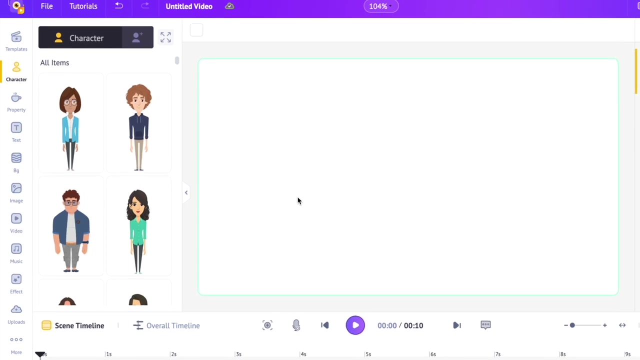 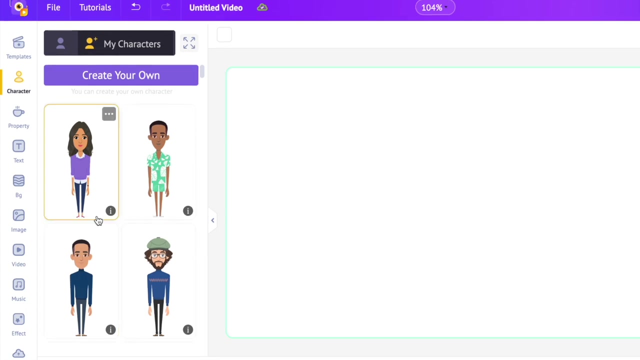 characters, starting from adult male and female characters, plus sized characters, animal characters and kids characters. To create a custom character from scratch, you have to open the my character section of the library. Here you are looking at all the custom characters that I have created before. To create a new custom character, 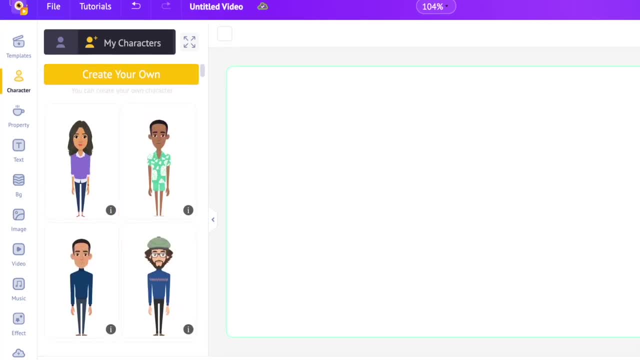 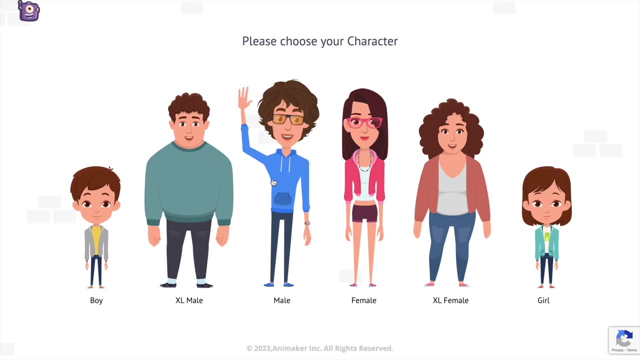 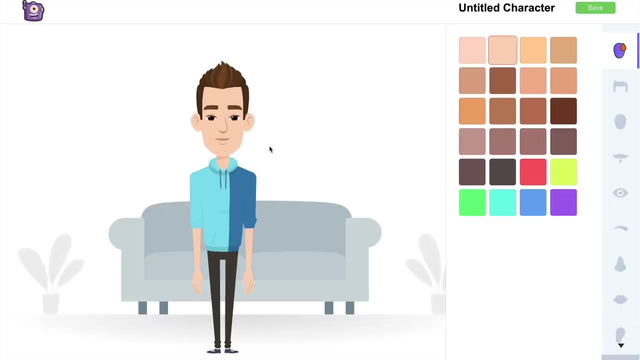 you should have to click on this option. create your own Now select the type of character that you want to create. Let me select the adult male character. Now we can start building the character, starting from the skin tone. Let's see the image of the character. 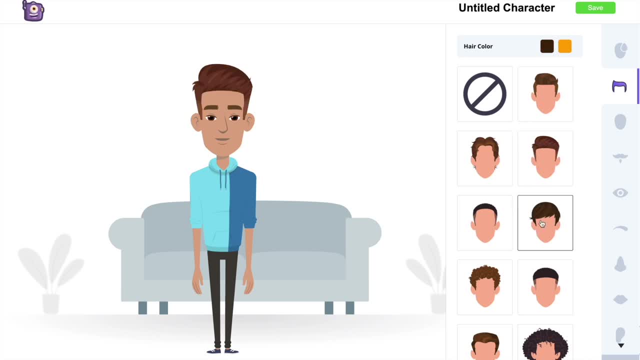 Next, we can see the different hair styles. we can also change the color of the hair. Following that, we have different facial features, like jawline, beard, style, eyes, eyebrows, nose, lips, ears and options to add wrinkles to the face. 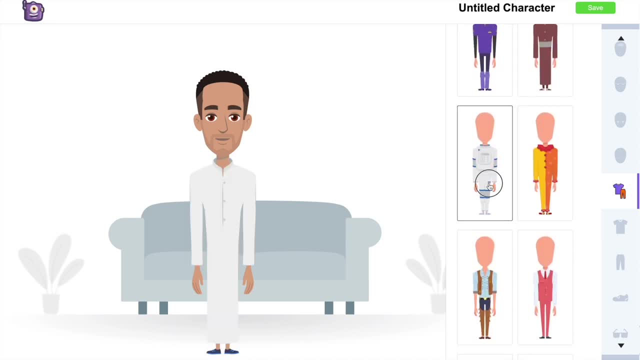 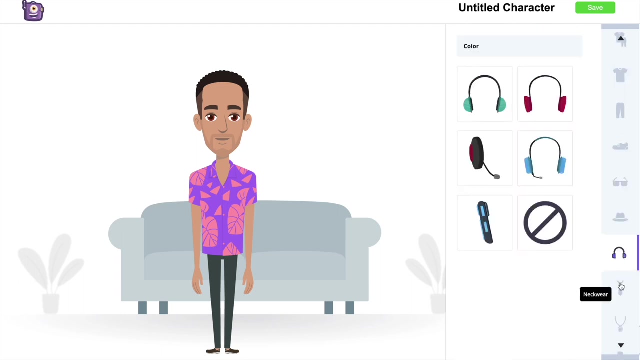 Next, we have the attire section. we can see attires of various nationalities and professions, Not by that, or the other elements like shoes, glasses, hats, headphones, etc. You can create billions of unique looking characters using all these options. Once all the changes are done, we can save the character using the option at the top. 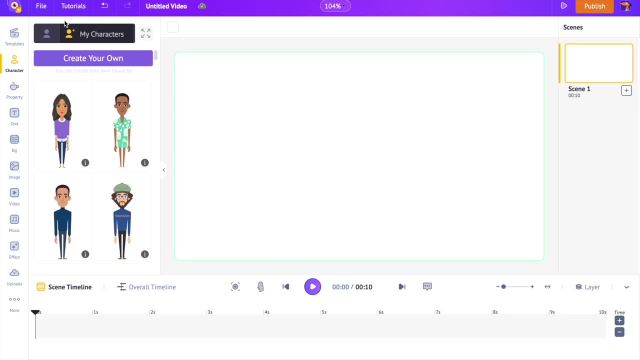 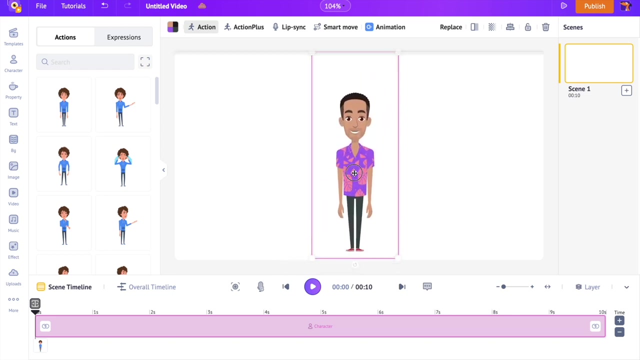 To use the saved character, we have to get back to the project Now. switch between the default character library and the my characters section. the created character will appear. Once you click on it it will appear on the workspace. We can resize and reposition the character anywhere within the workspace. 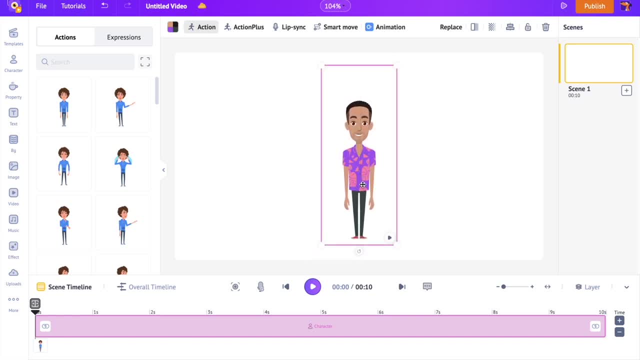 So that is how you can build a custom character easily, a comparatively easier method than drawing a character. In the upcoming part of this video, we will see how to animate this character, But before that, let's create a background for this scene. 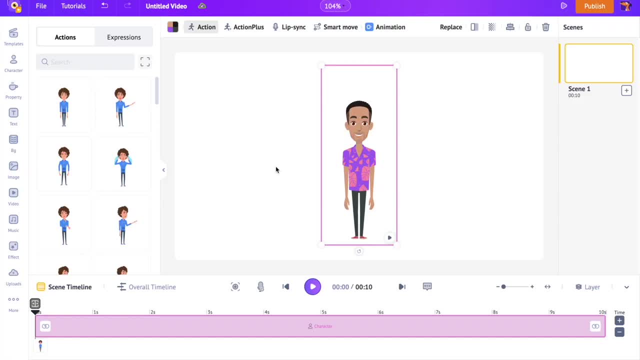 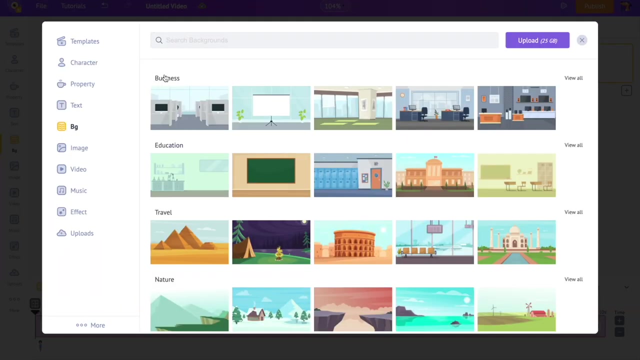 Step 2.. Creating a background. Drawing a detailed 2D background is difficult. That is why we are going to see how to add a background. Open the background section of the library. Here you can find different categories of 2D backgrounds, starting from business education. 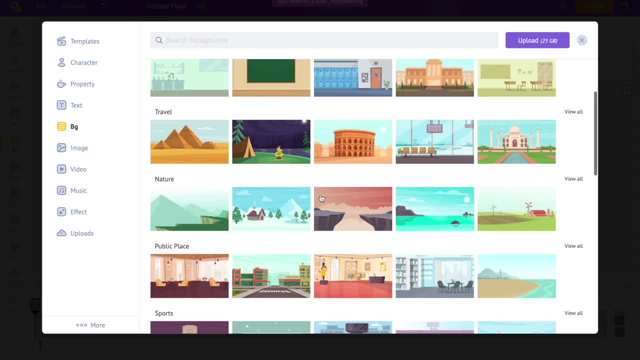 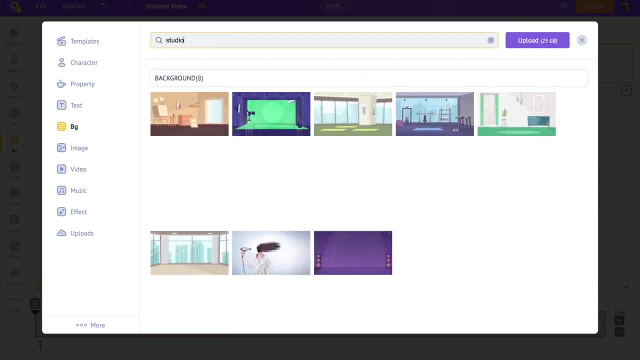 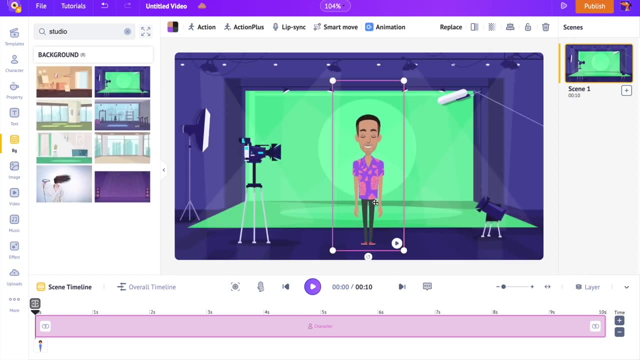 travel, nature, etc. We can also use the search option to find a background. Click and add the background to the video. It's time to animate the character- Step 3. Animating the character. An animation video works similar to a flip book. 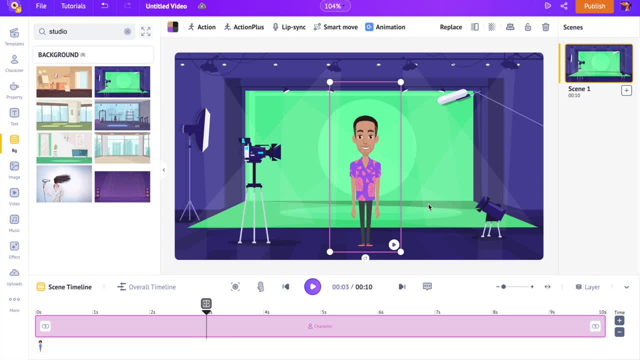 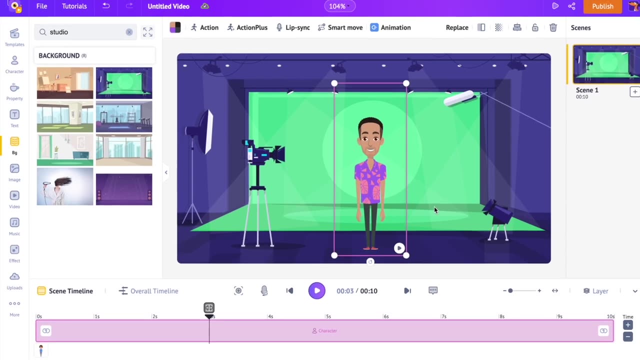 Similar to how you draw each page of a flip book. you have to draw individual frames which together become an animation video. But in our case we are going to replace this whole process of frame by frame animation with an option called action With the character selected. you can find it right above the workspace. 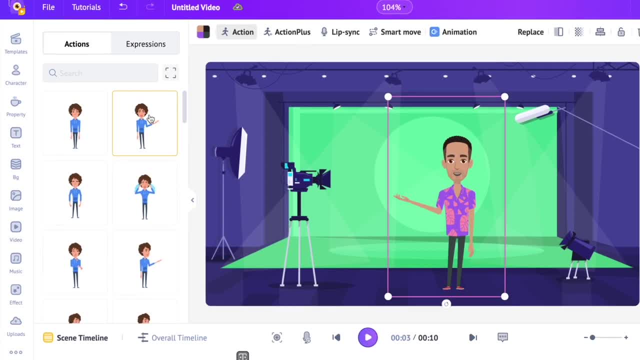 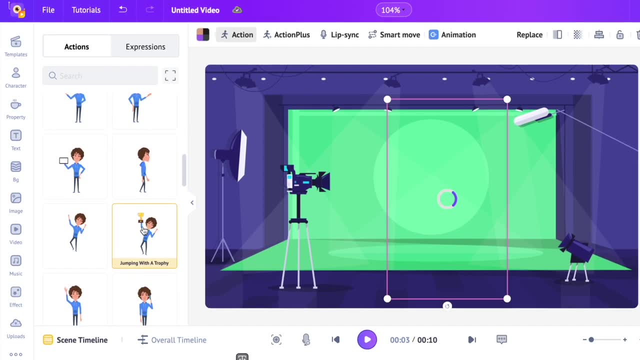 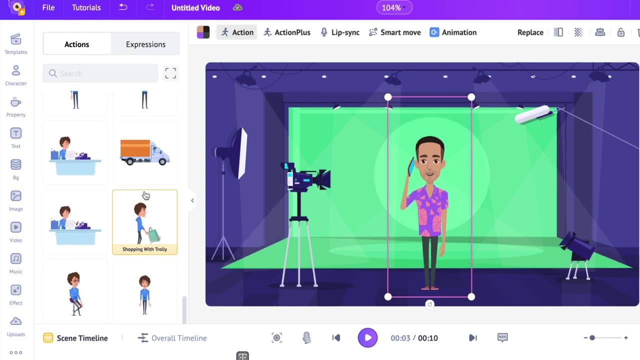 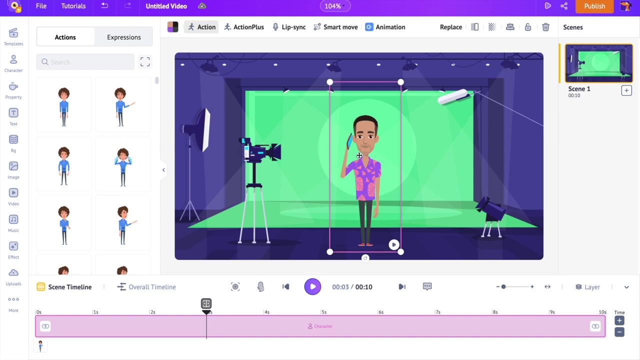 Let's try out a few of these actions. Consider each of the actions as an animation loop. There are more than 800 different actions that you can apply to a character. By adding multiple actions to a character, we can animate it. For example, in this video, I want the character to walk into the scene then greet the audience. 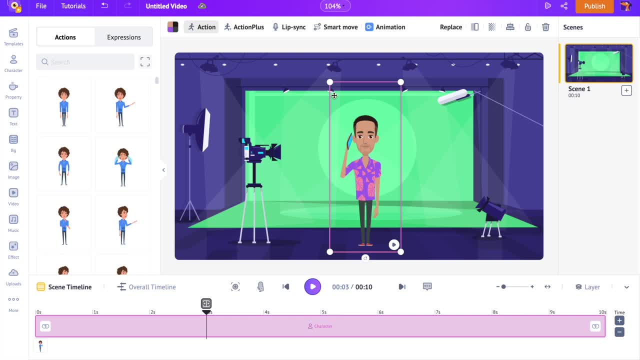 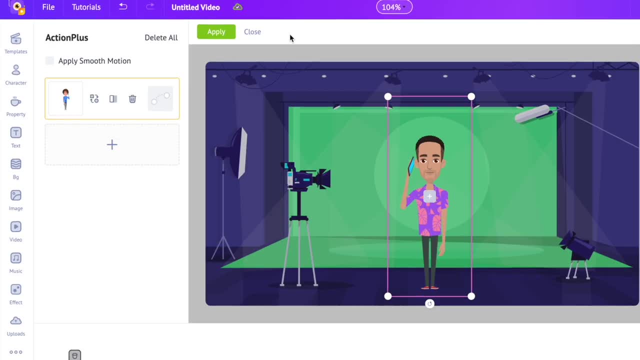 and then it should start talking. So the character has to perform three different actions one by one. To add multiple actions, we have to use the action plus option over here. Let's start with a walking action. We can see a lot of different walking actions in the results. 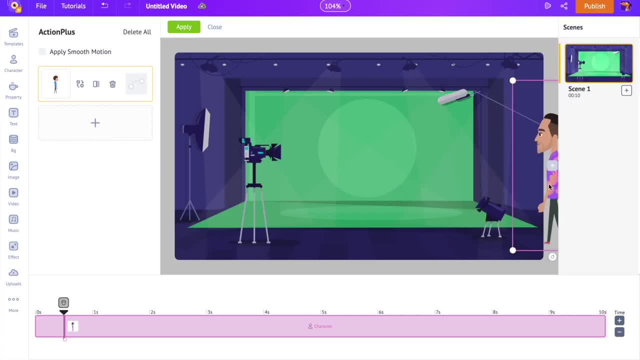 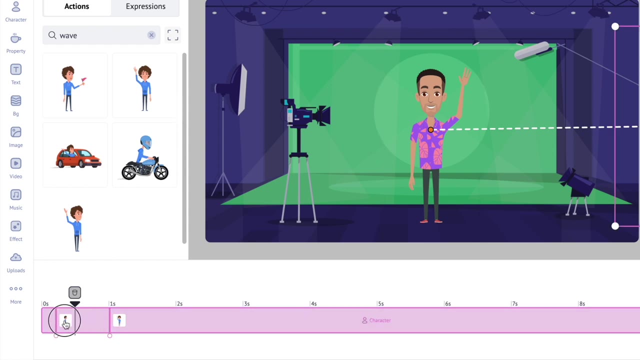 Let me select this one over here To add the next action. We have to use the plus icon over here On the timeline we can see thumbs. They represent each of these actions that we have added down. By moving them we can control the time duration taken between each action. 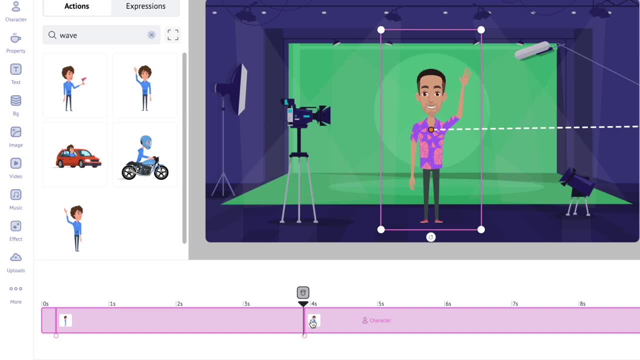 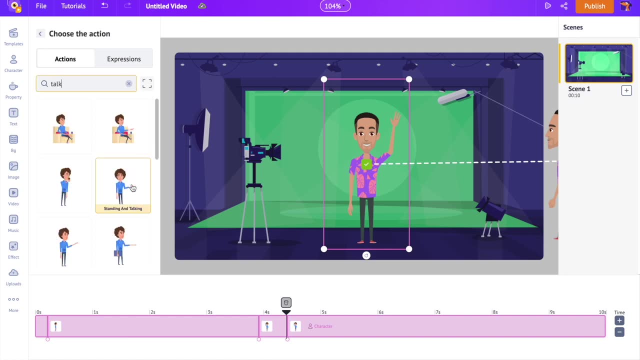 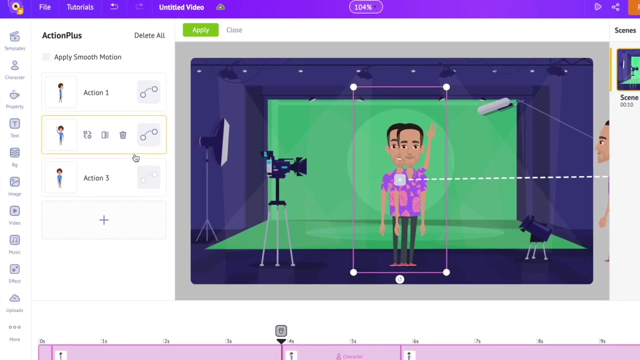 I'm giving around four seconds between the first two actions. I'm adding a talking action as a third one And I'm giving two seconds between the second and the third action. For a smoother transition, make sure to select the icons present over each of the actions. 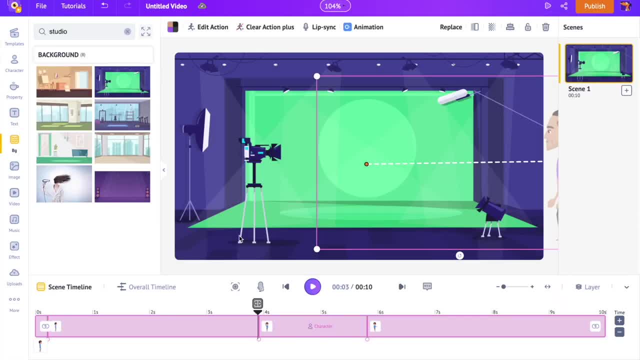 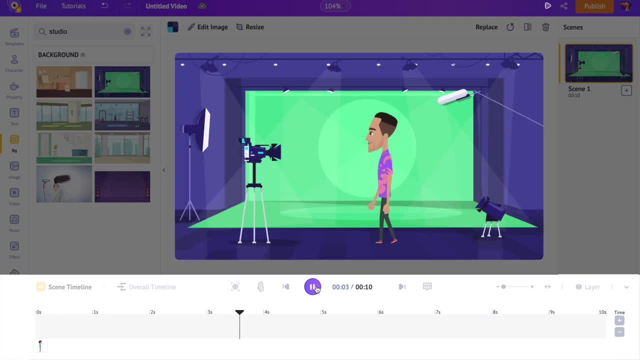 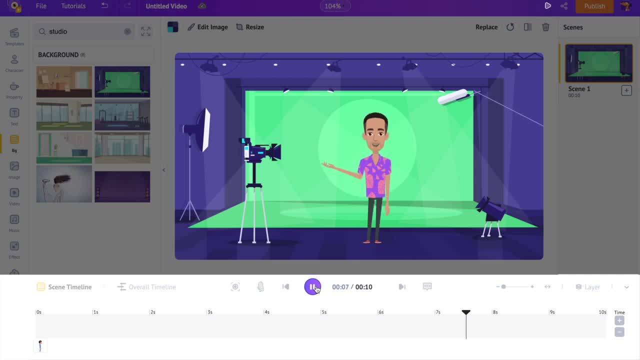 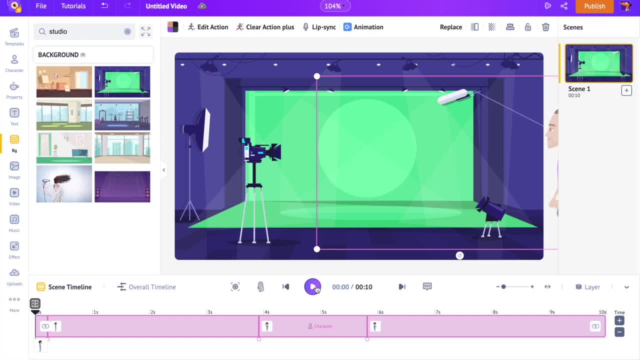 We animated the character in just under four minutes, which probably would have taken us a few hots through the regular animation method. If this is exciting to you, then you'll be more excited to know how to add lip sync voiceovers to these characters. 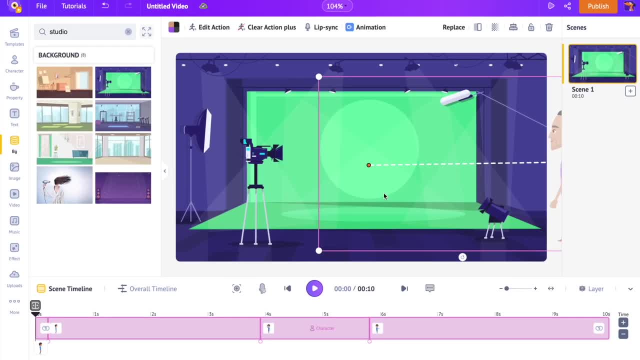 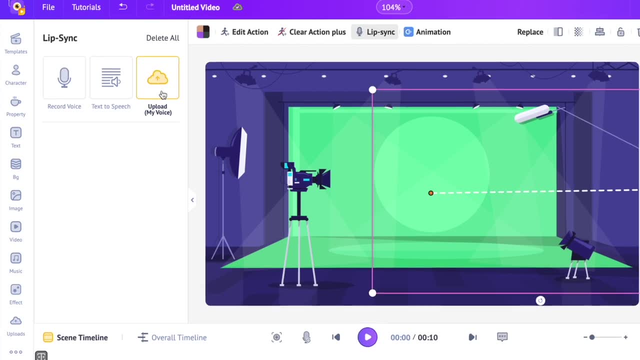 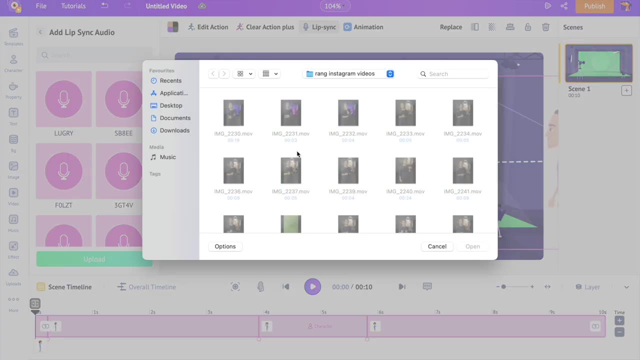 Step Four: adding voiceovers with lip sync. With the character selected, click on the lip sync option present about the workspace. Now you'll get three different options to add the voice over. On the right have the option to upload pre-recorded audio files. let's say you have an audio file that you want to. 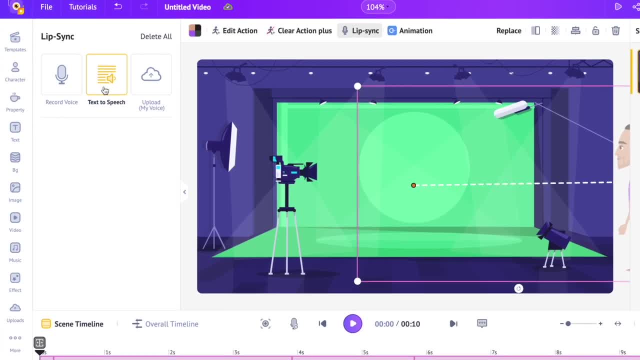 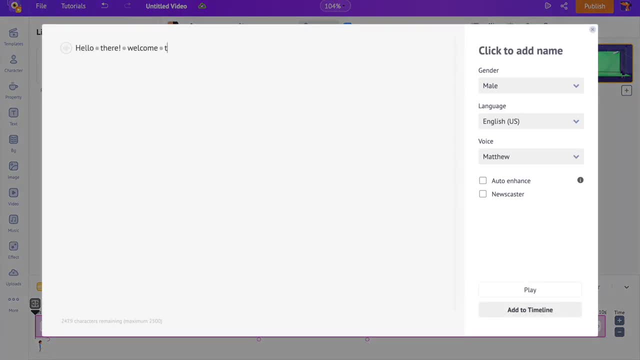 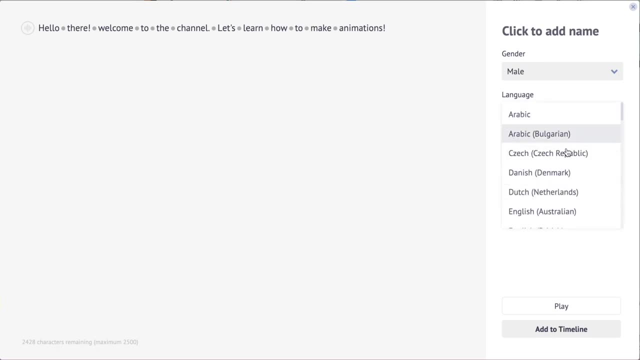 add as a voiceover, then this is the option that you have to use. in the middle is the text to speech option. this will convert any text into audio and add it as a voiceover. after typing the text, you have to choose the options on the right hand side, starting with agenda. then we have the 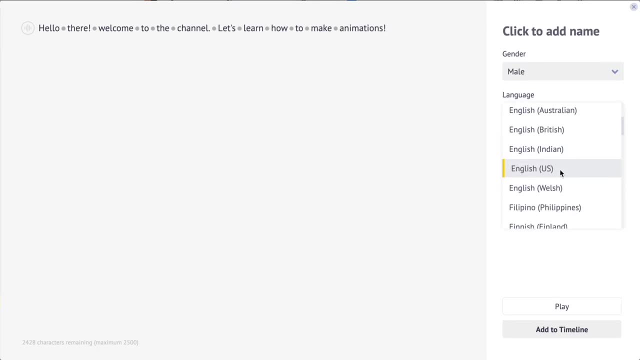 option to choose a language. then we have the option to select among a list of voices. hello there, welcome to the channel. let's learn how to make animations. you can further customize the audio using the options over here. you can control the speed, pitch and the volume of the voice. you can also add break and breathing effect between the words. 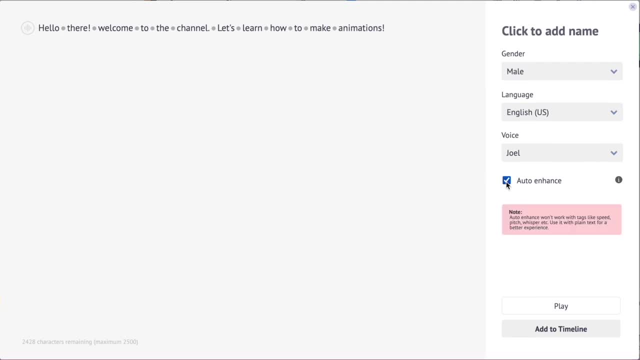 this auto enhance feature will make the audio human-like in a single click. this feature is available for premium users. hello there, welcome to the channel. let's learn how to make animations. once you click on the add to timeline option, the voiceover will be added to the video. 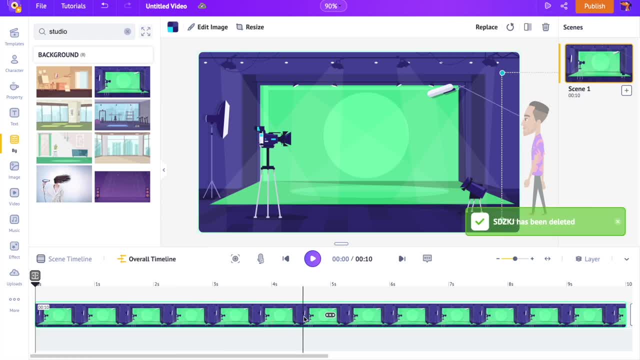 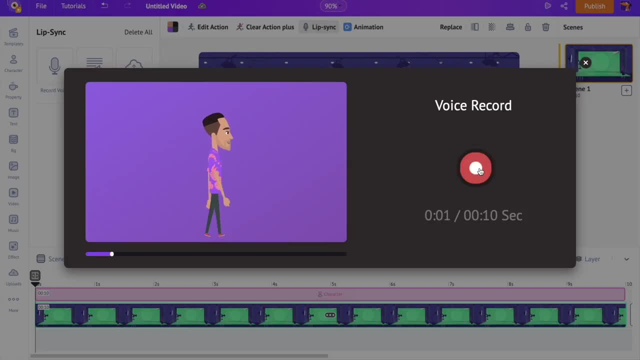 but for our animation video we'll be using the first option, that is, the record voiceover option. let's record the voiceover. hello there. welcome back to the channel. let's learn how to make animation videos. here you can preview the recorded voiceover. you can re-record the voiceover if required or apply it to the video. 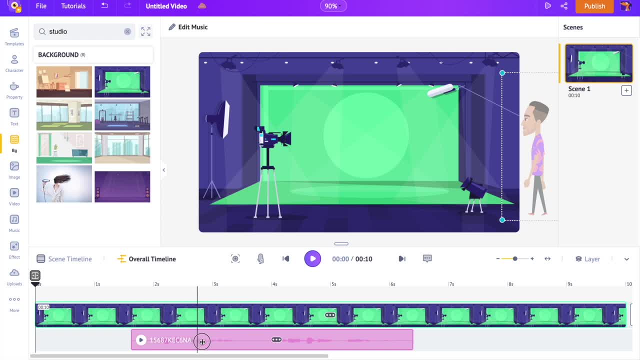 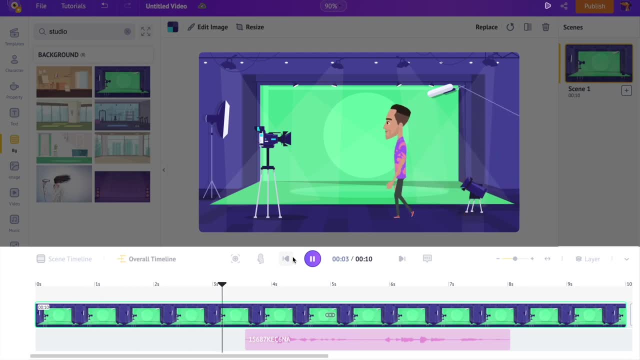 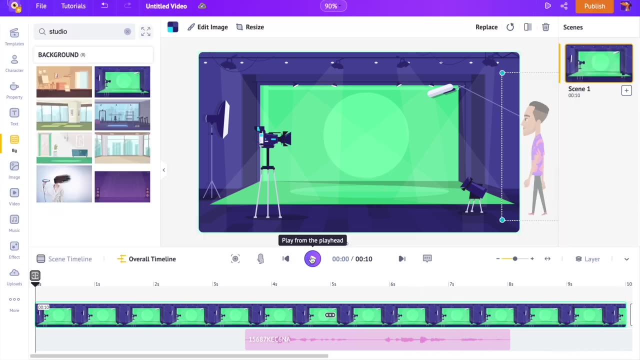 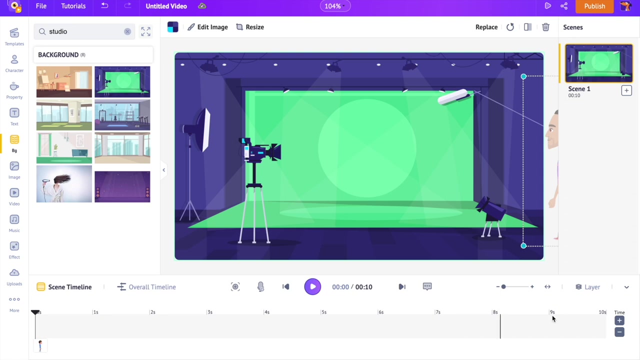 let's adjust the position of the voiceover on the timeline to match the actions of the character. hello there. welcome back to the channel. let's learn how to make animation videos. we can see that there is some extra duration on the scene. to add or remove the duration you have to use the plus and the minus. 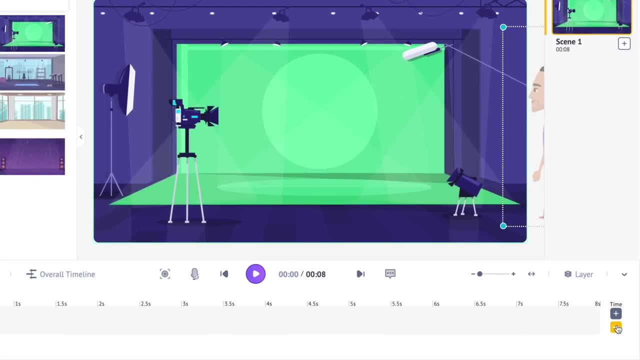 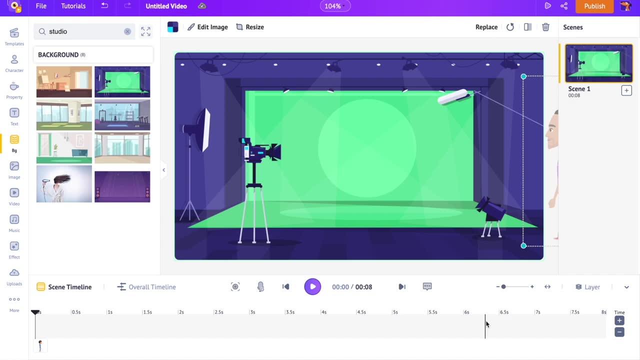 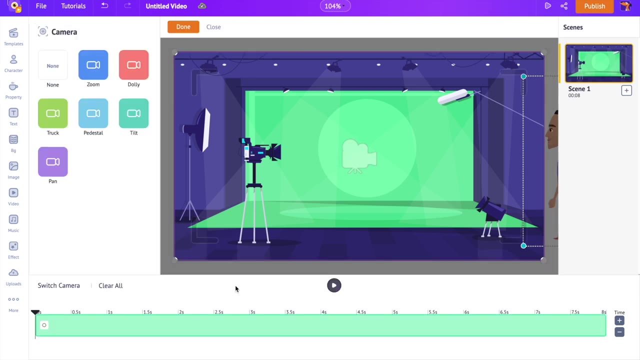 option present at the bottom of the scene timeline. i have reduced the scene duration to 8 seconds. as the next step, let's see how to add camera effects like zoom in and zoom out, to the scene. step 5: adding camera moments. to add a camera effect: open the camera timeline.